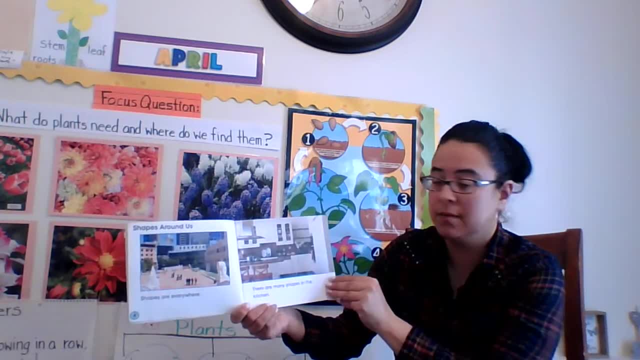 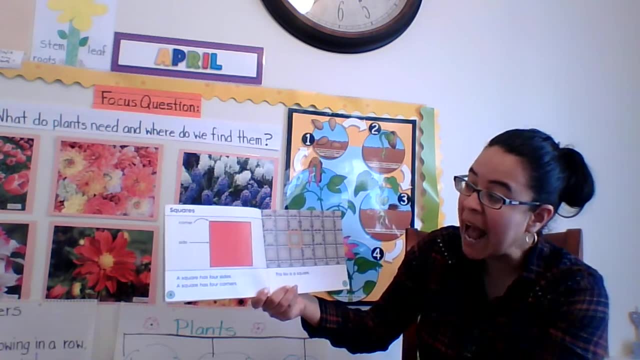 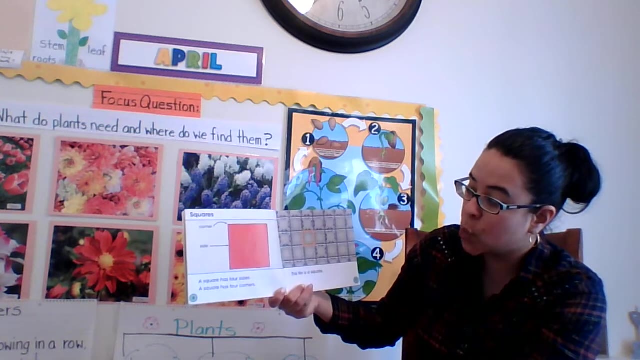 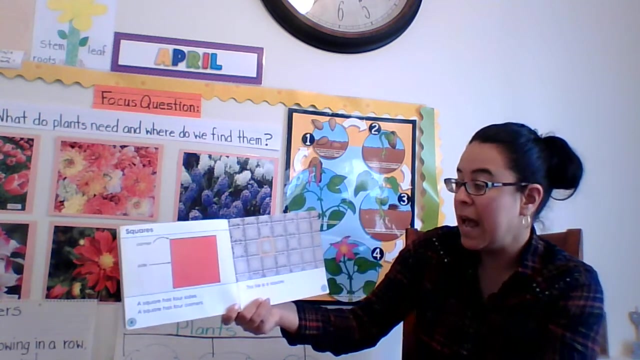 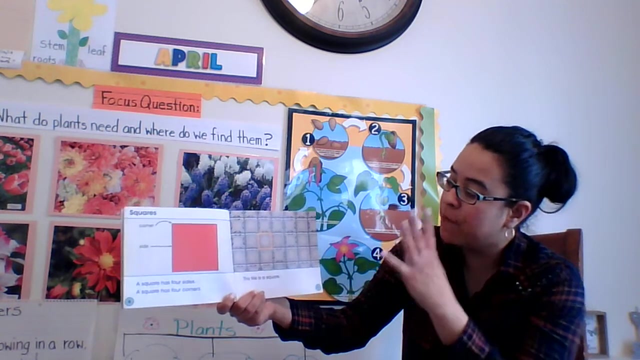 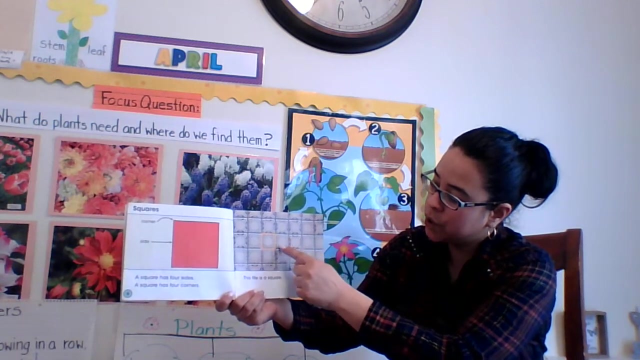 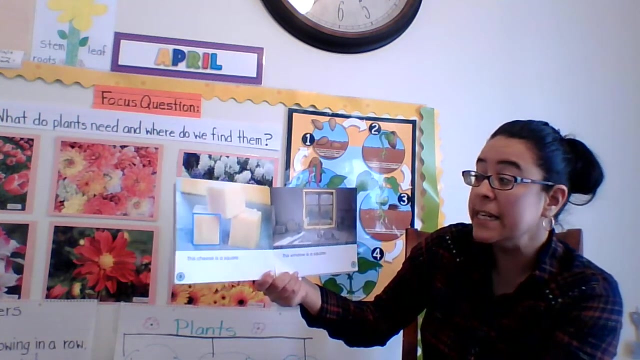 what shapes can you find in your kitchen? squares? a square has four sides: one, two, three, four. a square has four corners: one, two, three, four. this tile is a square because it has four sides right and four corners: one, two, three, four sides. one, two, three, four corners: this cheese is a square. 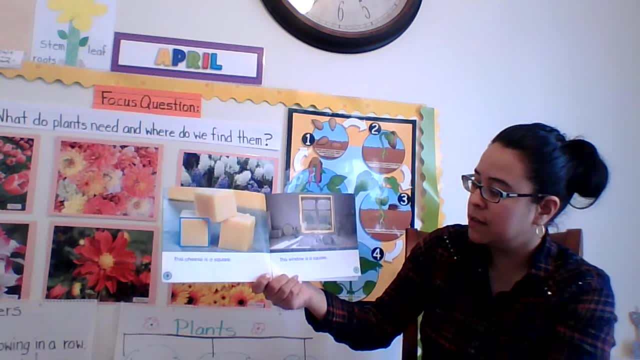 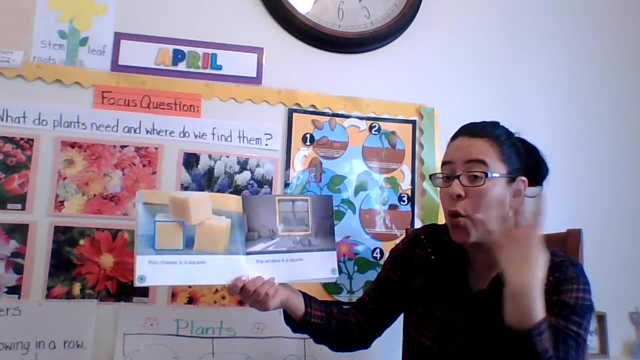 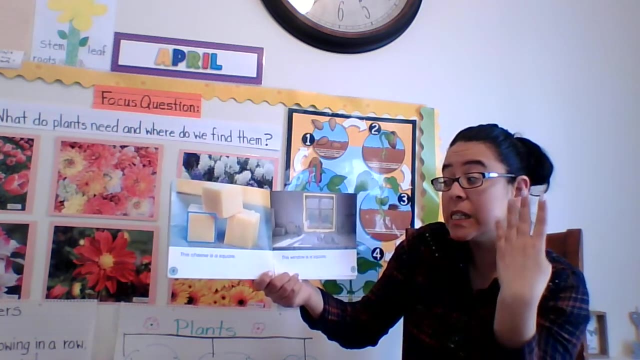 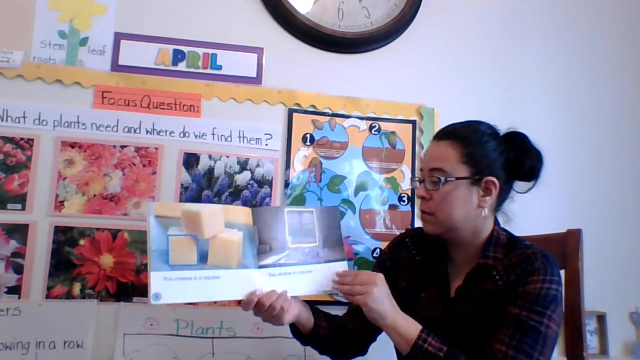 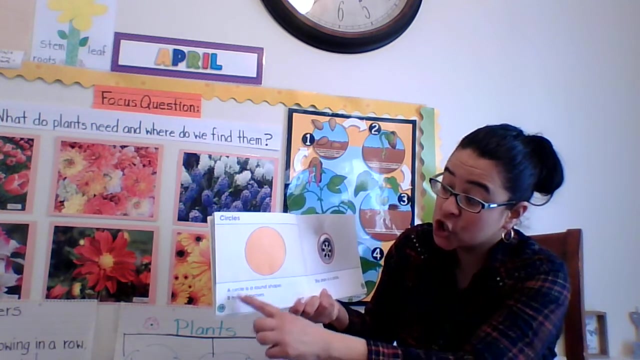 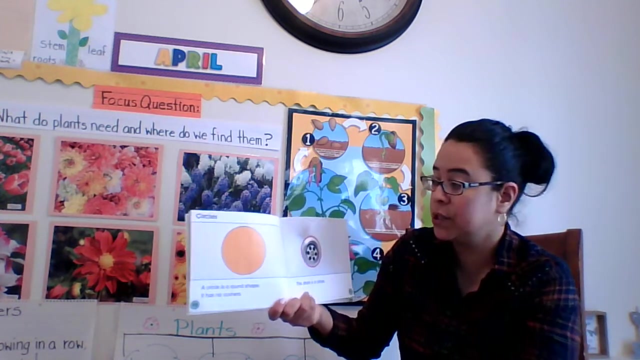 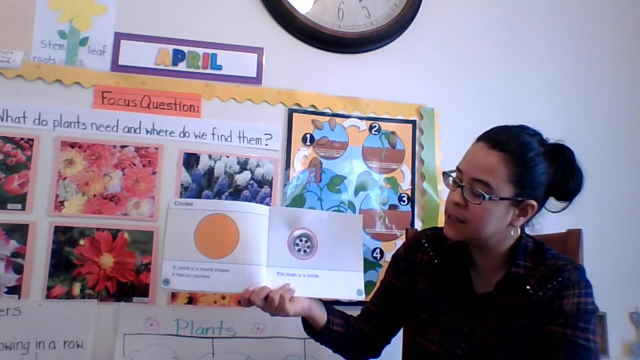 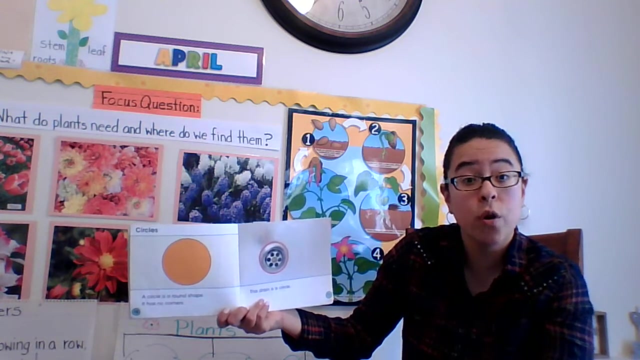 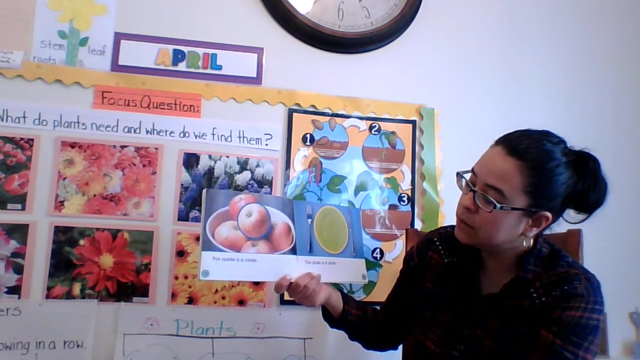 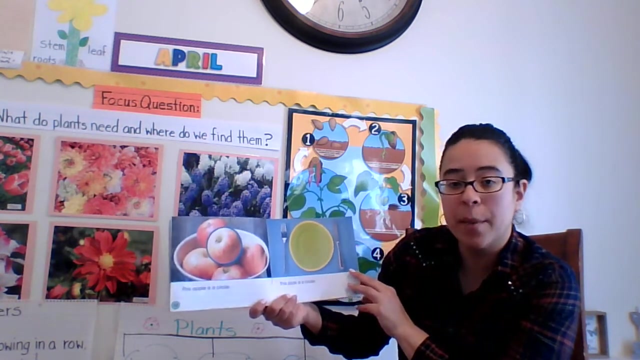 this window is a square because it has what? four sides and four corners. very good, one, two, three, four, four sides. one, two, three, four, four corners, circles, okay, a circle is a round shape, it has no corners. the drain is a circle because it has how many corners? no corners, zero, zero corners. good, this apple is a circle and circles have how. 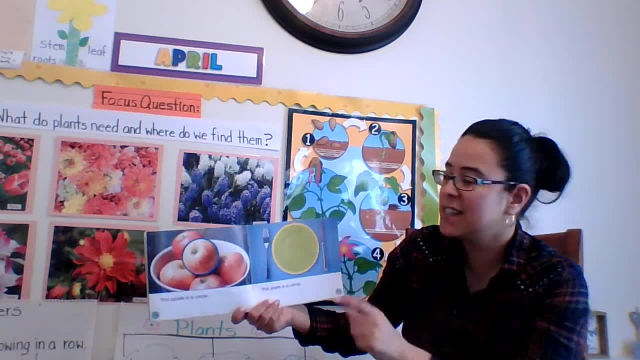 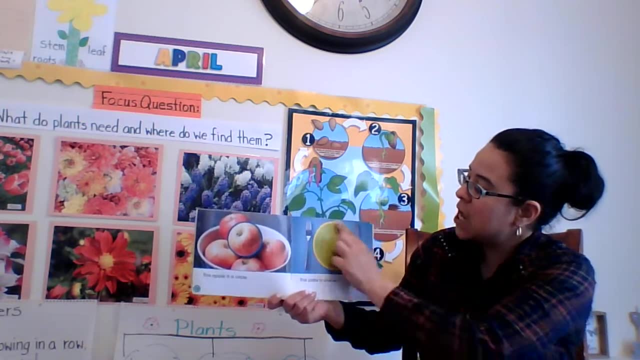 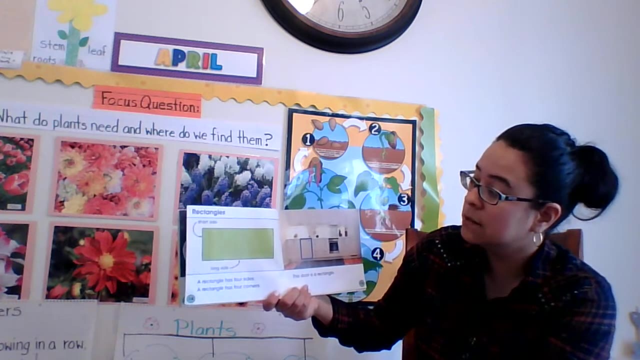 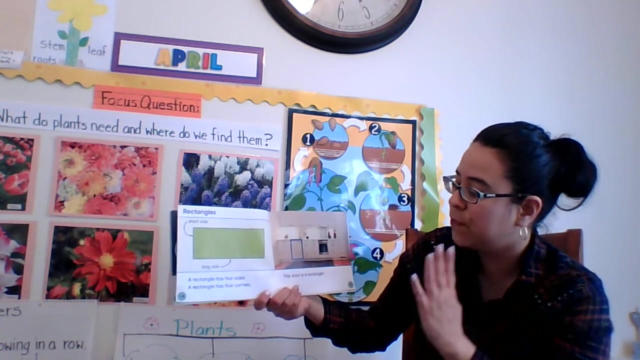 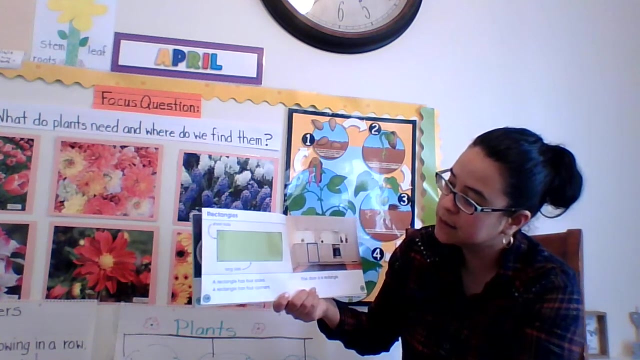 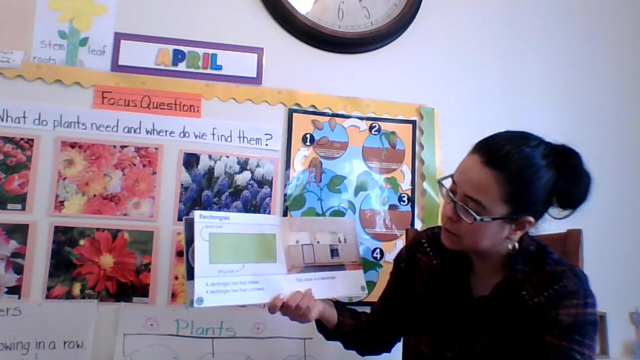 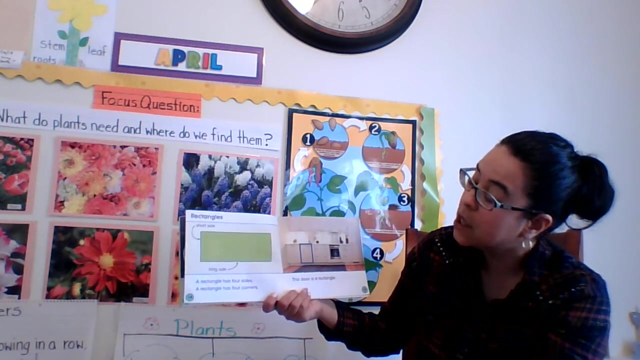 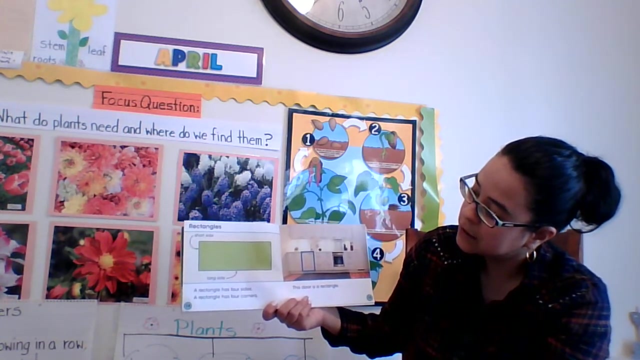 many corners? zero, good, zero corners. this plate is a circle. it goes round and around and around rectangles. a rectangle has four sides. a rectangle has four corners. that's one, two, three, four sides and four corners: one, two, three, four. you, these sides are a little different than a square here. these are parallel, two long. 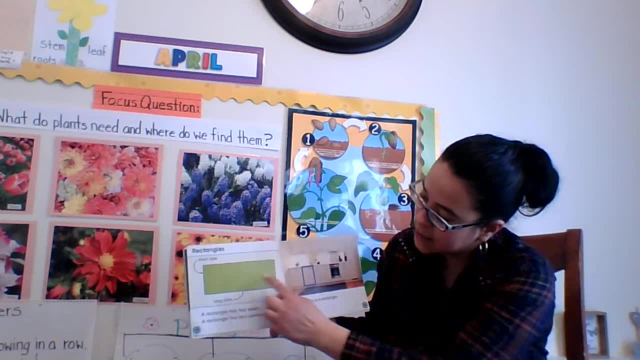 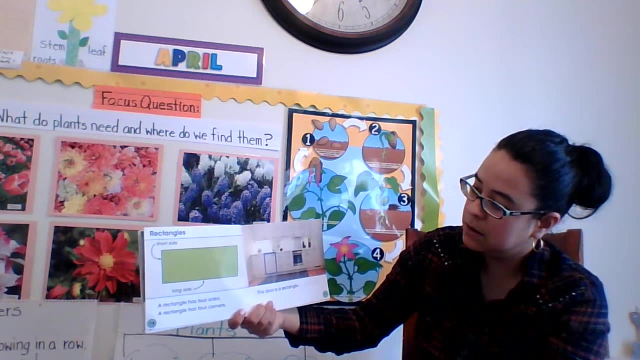 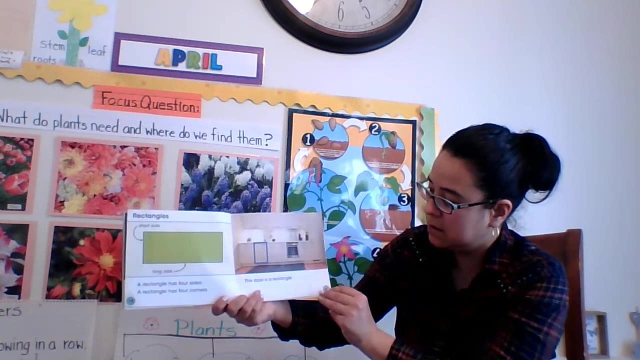 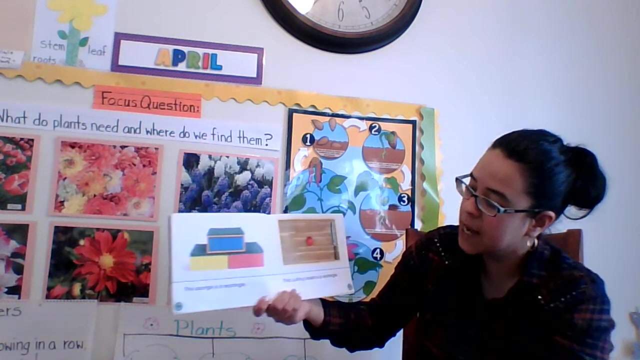 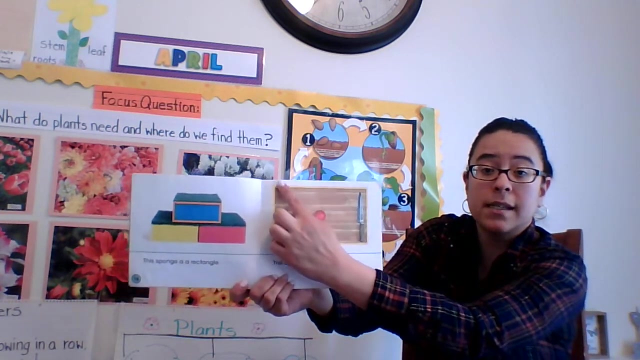 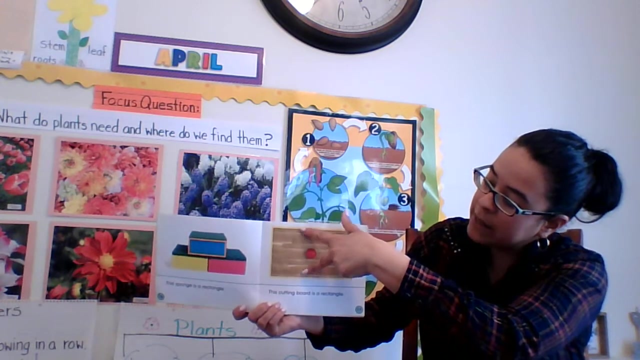 sides that are parallel to each other, and these sides here are the short sides that are parallel to each other. okay, they're not the same length. this door is a rectangle. this sponge is a rectangle. this cutting board is a rectangle: four sides, four corners. has two parallel long sides, two parallel short sides. 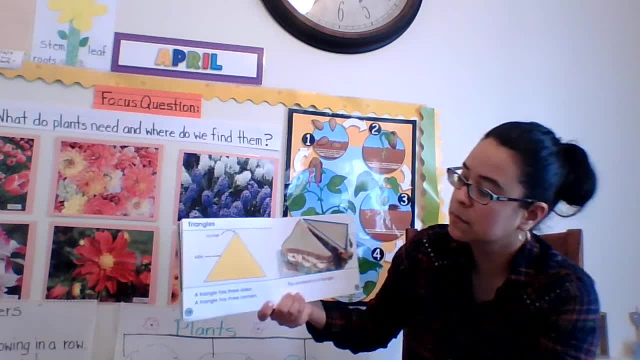 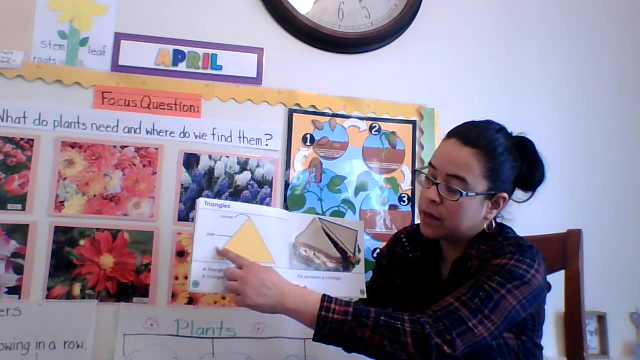 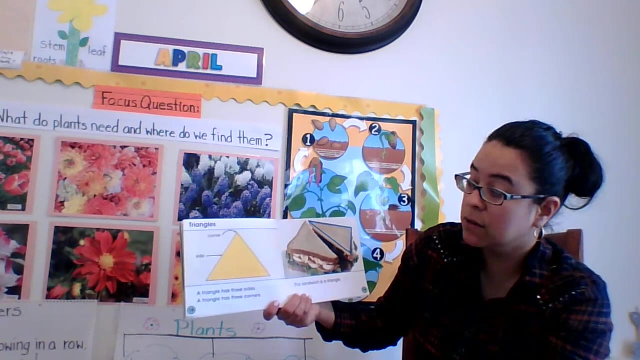 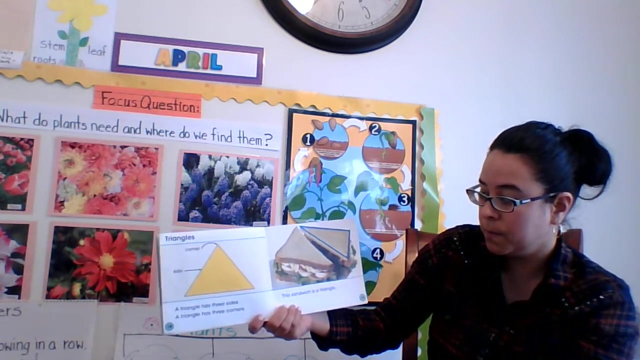 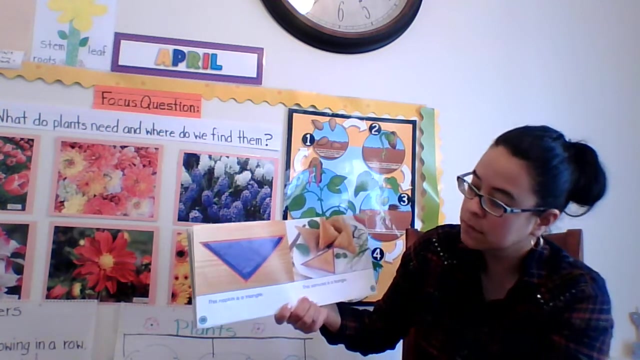 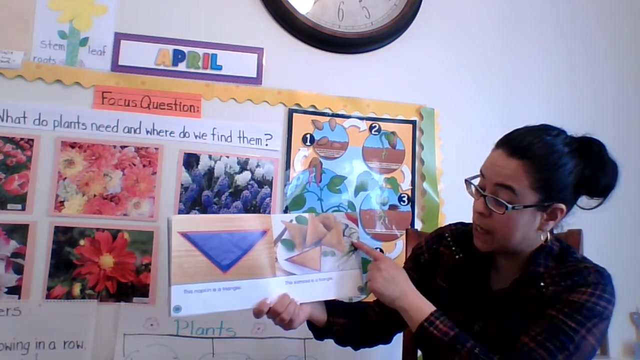 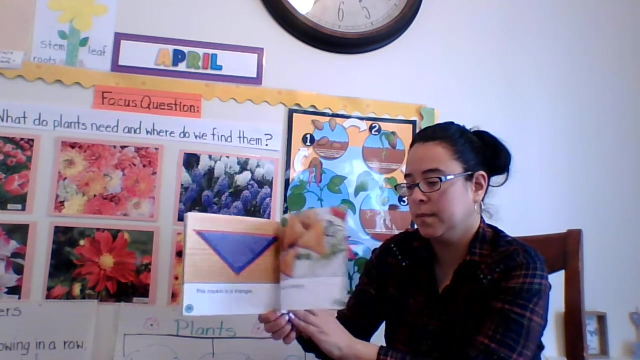 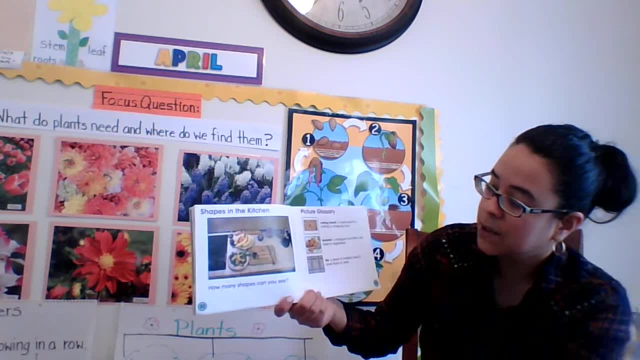 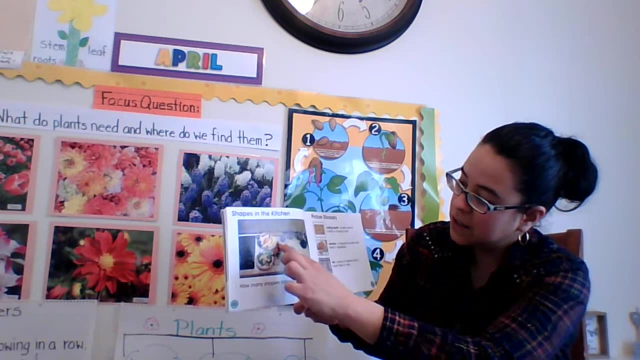 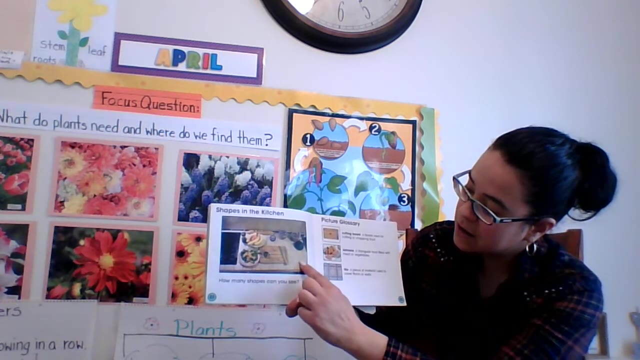 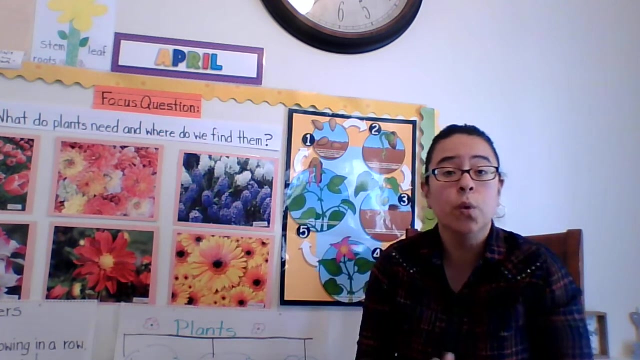 we have here rectangular Circle Circle. There's a bowl, another circle: You have these tiles here, right? that are squares. All right, boys and girls. So what you can do at home with your family is play a game, okay. 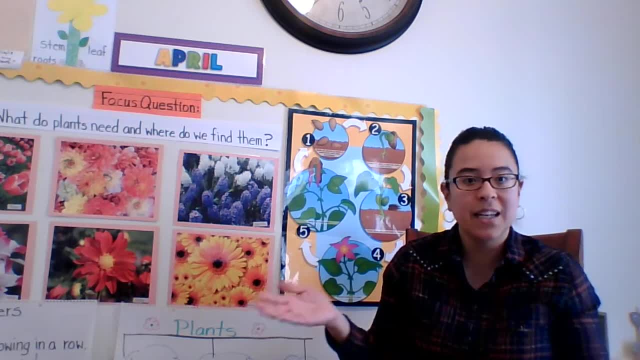 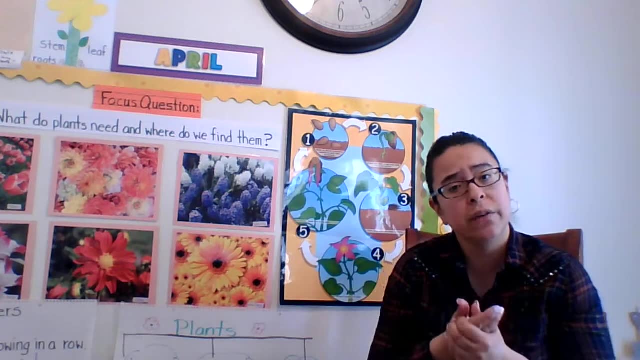 Have you heard of the game I Spy? I think so. I think we've played this game before I Spy, So you can go around your home, your kitchen, your living room, your bedroom, dining room and look for shapes, okay. 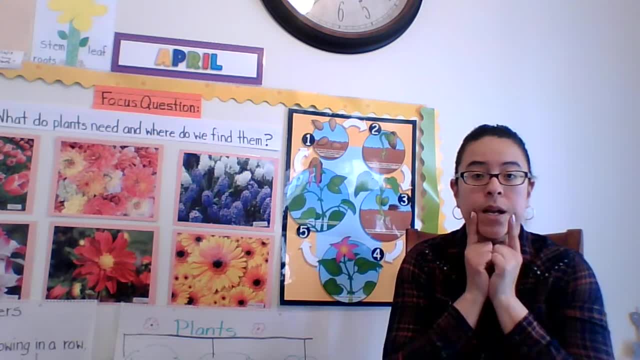 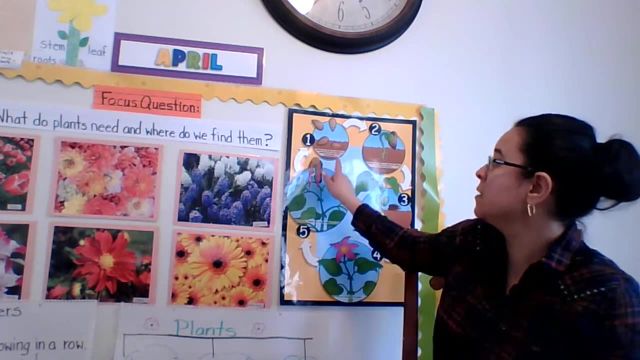 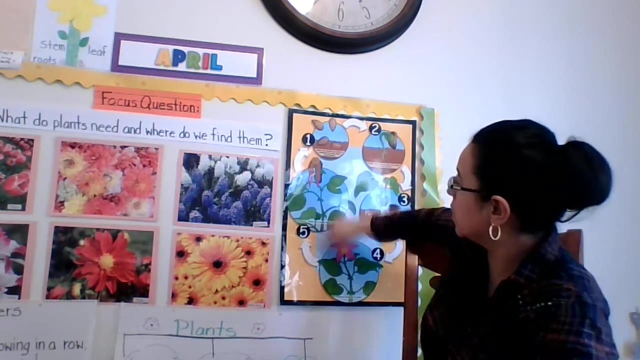 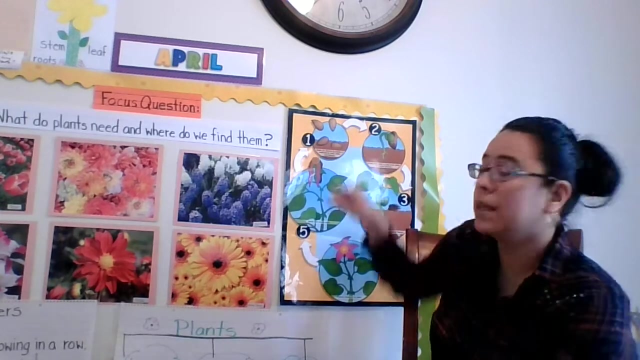 You can look for shapes. Let me see. I spy a rectangle behind me. This poster has four sides. too long, too short, They are parallel. These long sides are parallel to each other. These short sides are parallel to each other.